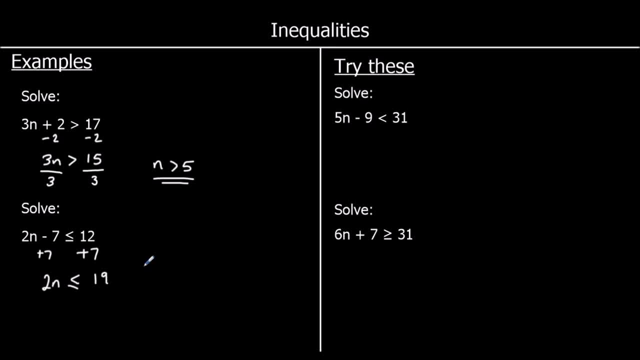 that times 2.. So do the opposite of times n by 2,, which is dividing by 2.. So I'm going to divide both sides by 2.. So I'm going to get rid of that times 2.. So I'm going to. 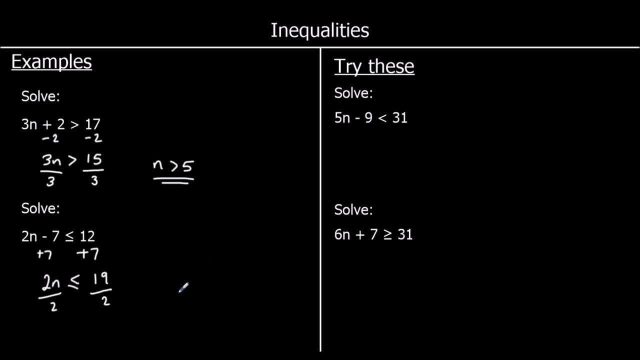 divide both sides by 2. And the answer is: n is less than or equal to 19 over 2.. Or, if you want to write that as a decimal, that'll be 9.5.. Okay, two questions for you to try. So pause the video and give them a go. 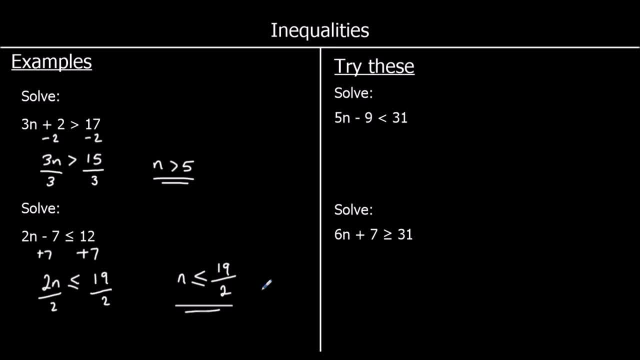 Okay, the first one we've got: 5n minus 9 is less than 31.. So I'm going to get rid of minus 9.. So the opposite of minus 9 is plus 9.. So I plus 9 to both sides, which leaves: 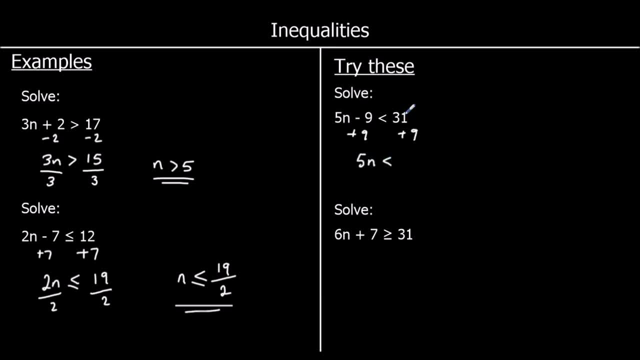 me with 5n is less than 40.. 31 plus 9 is 40. So I've got n times 5 at the moment is less than 40. To get n by itself, do the opposite of times n by 5.. Divide by 5.. So that leaves. 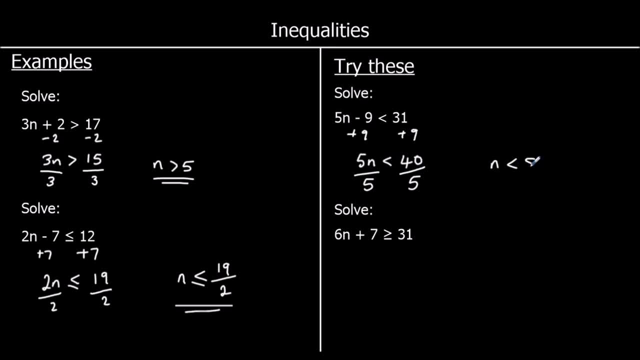 me with n is less than 8.. And the second one, 6n plus 7, is bigger than or equal to 31.. I'm going to get rid of plus 7 by minusing 7 from both sides, So I've got 6n is bigger. 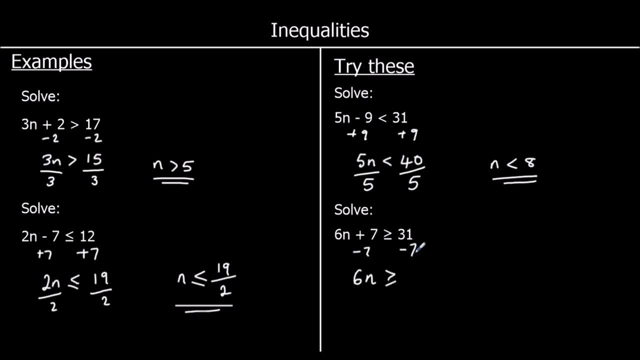 than or equal to 31, take away 7,, which is 24.. So n is times by 6. at the moment, To get rid of a times by 6, I'm going to divide both sides by 6.. So n is bigger than or equal to 24 over 6,, which is 4.. 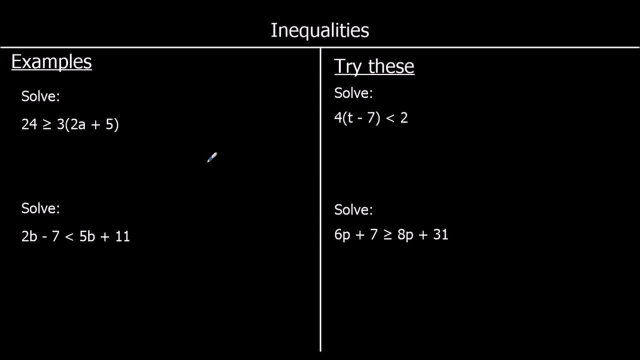 Okay, another couple of examples. We're going to again just follow the steps of solving equations, Doing the same to both sides. So I'm going to expand this bracket first. So I'm going to leave 24 as it is. It's bigger than or equal to. I'm going to expand the bracket. 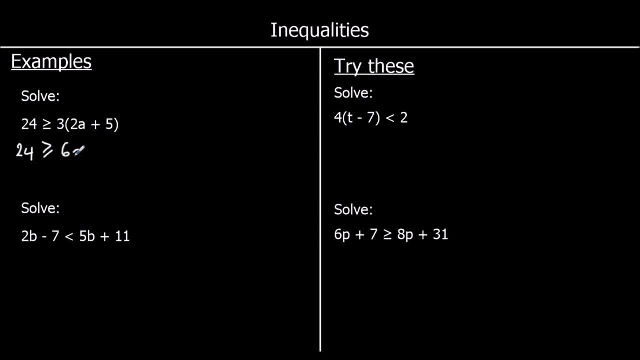 So 3 times 2a is 6a And 3 times 5 is 15.. So I want to get a by itself. I'm going to start by taking away 15 from both sides. So I've got 6a plus 15 at the moment. To get rid of a plus 15, I'm going to take away 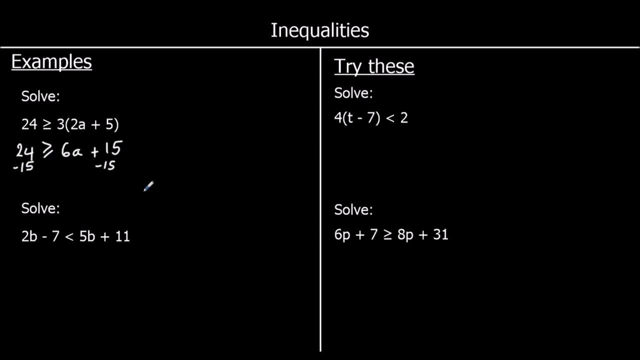 15.. So 24 minus 15 is 9.. So I've got: 9 is bigger than or equal to 6a, And a is times 6 at the moment. So I'm going to divide by 6,, divide both sides by 6.. So 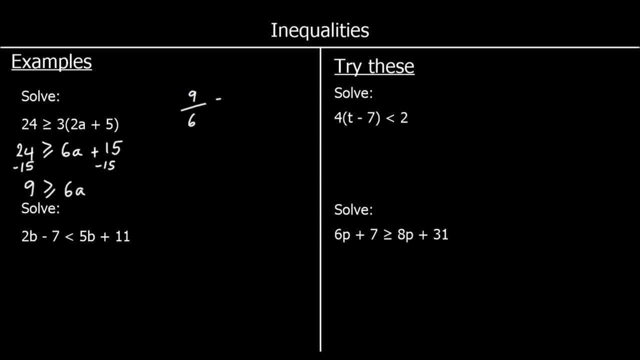 9 divided by 6.. 9 divided by 6 is bigger or equal to 6a over 6, which is a, And I can simplify: 9 over 6.. They're both in the 3 times table, So that's 3 over 2.. 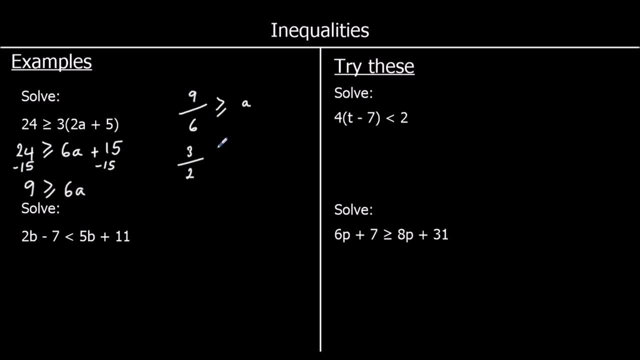 9 is 3, 3s, 6 is 2, 3s. So 3 over 2 is bigger or equal to Теперь a, and if i want to write a first, a is on the smaller side. a is less than or equal to 3 over 2. 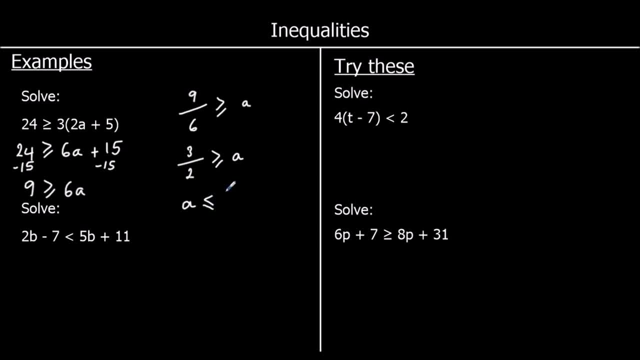 so i can just write: a is less than or equal to 3 over 2, and if i wanted to write that as 1.5 as well, i could. the second one: i've got an unknown on both sides. i've got 2b on the left side and 5b on the right side. 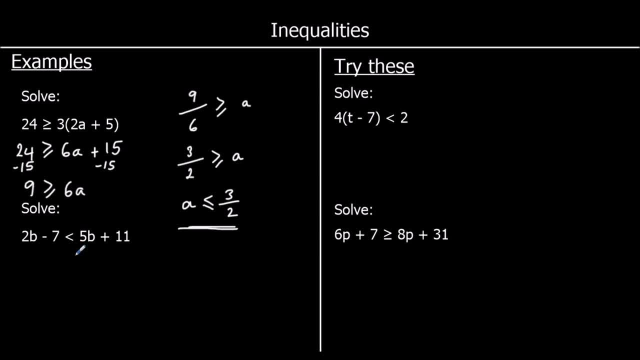 i'm going to start by getting rid of the smallest b, so i'm going to take 2b away from both sides. 2b is less than 5b, so i'm going to get rid of that one first, which will leave me with a positive b. 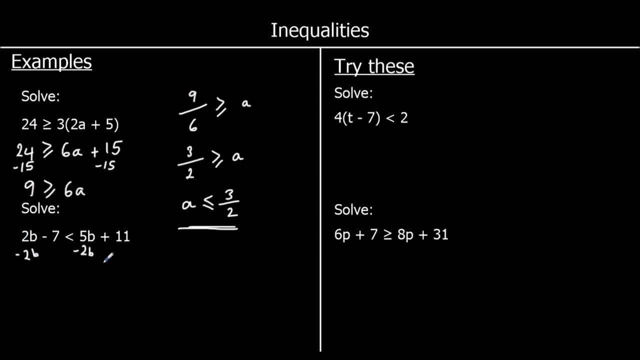 so if i take 2b away from both sides, on the left side i've got 2b negative 7 left. the sign is less than so negative 7 is less than 5b. take away 2b, which is 3b plus 11.. 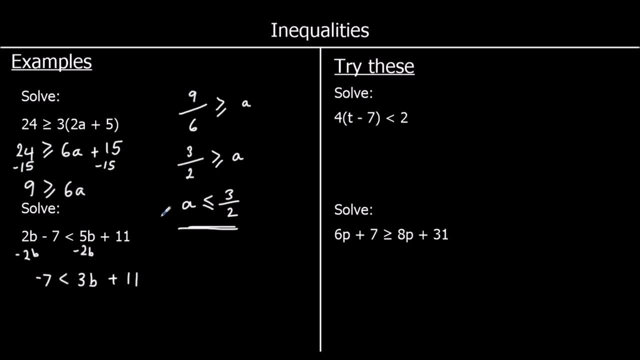 so i want to get b by itself. i'm going to get 3b by itself to start with, so i'm going to take away 11 from both sides. i've got minus 7, negative 7. take away 11 which is negative, 18. negative 18 is less than 3b and i'm going to divide both sides by 3. 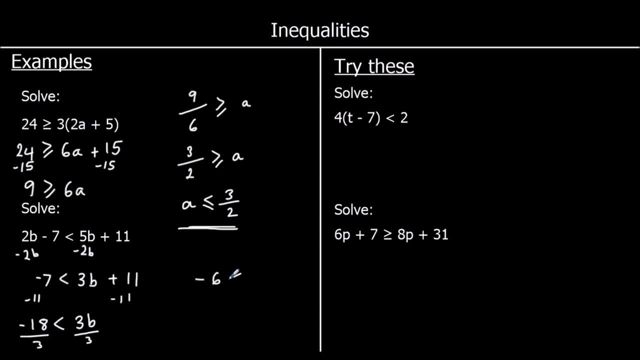 which gives me negative 6 is less than b. if i want to write b at the front, b is on the bigger side, b is bigger than negative six, so i can just rewrite it as b is bigger than negative six. okay, two for you to try. so pause the video and give them a go. 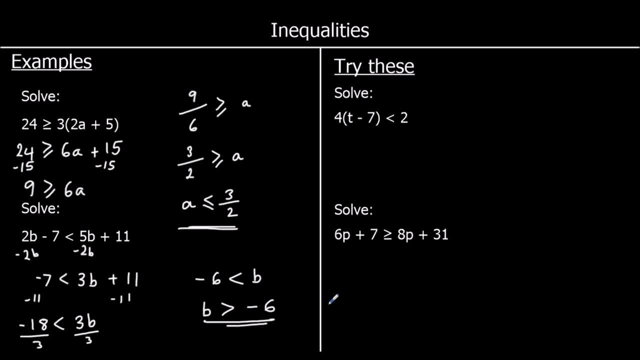 okay, the first one. i'll start by expanding the brackets. so 4 times t is 40. 4 times negative 7 is negative 28 and that is less than 2. i'm going to add a plus 28 to both sides, so that leaves me with: 40 is less than 2, plus 28 is 30, and then dividing both sides by 4, 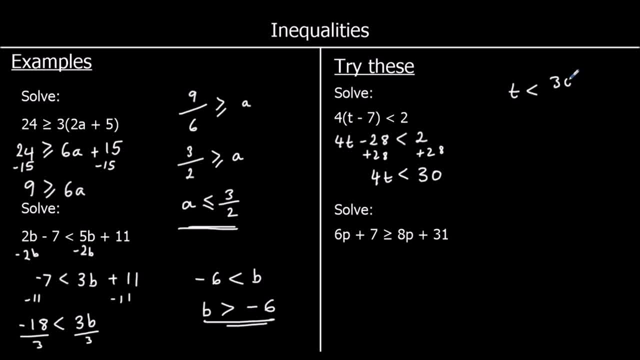 t is less than 30 over 4 and if i half top and bottom that will be 15 over 2. that's as simple as it gets. you could write it as a decimal, which would be 7.5, but a fraction is a perfectly good answer. 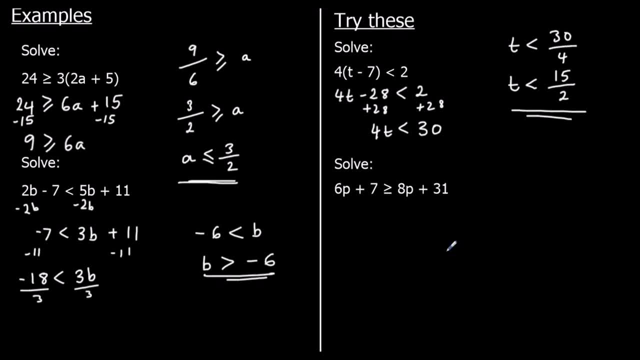 and the second one. i'm going to get rid of the smallest p first, so i'm going to take 6p away from both sides, which will leave me with: 7 is bigger or equal to 8p. take away 6p is 2p. 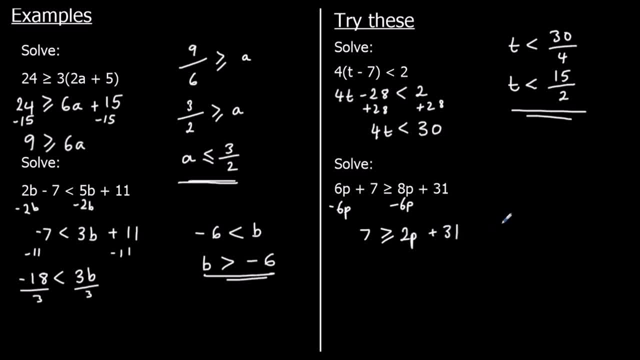 plus 31.. i want to get p by itself, so i'm going to take 31 away from both sides. 7 take away 31 will be negative. 24 negative 24 is bigger or equal to 2p halving both sides, or can be negative. 12 is bigger or equal to p. and if i want to write p on the front, 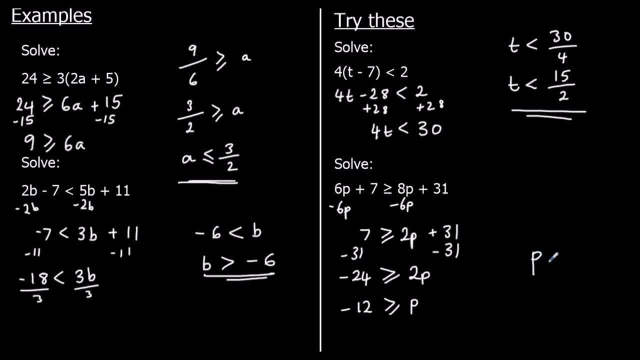 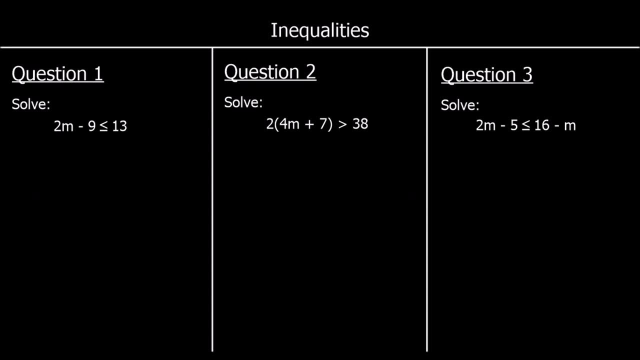 p is on the smaller side, so i can write: p is less than or equal to negative 12.. okay, three questions to finish up for you to try. so pause the video, give them a go and press play when you're ready for the answer. okay, question one solve: 2m minus 9 is less than or equal to 13.. 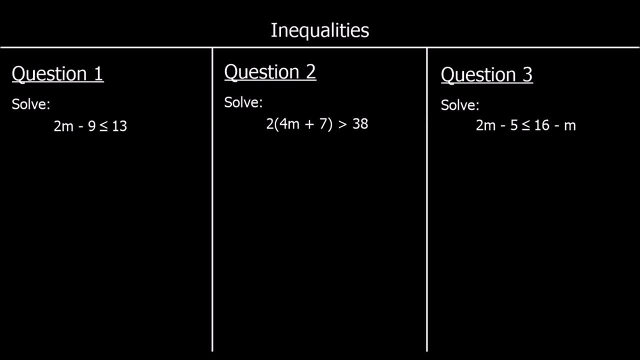 so we want to get m by itself. at the moment we've got a minus 9. to get rid of that, we'll plus 9 to both sides, so that will leave us with 2m is less than or equal to 13 plus 9. 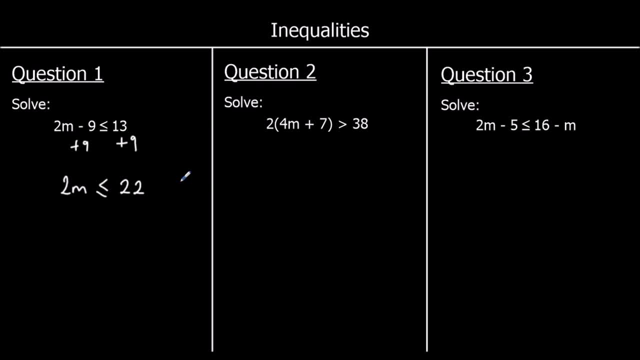 so 22.. to get m by itself, we're going to divide both sides by 2. so halving both sides gives us m is less than or equal to 11.. question two: we'll start by expanding the bracket. so 2 times 4m is 8m, 2, 7s are 14.. so 8m plus 14. 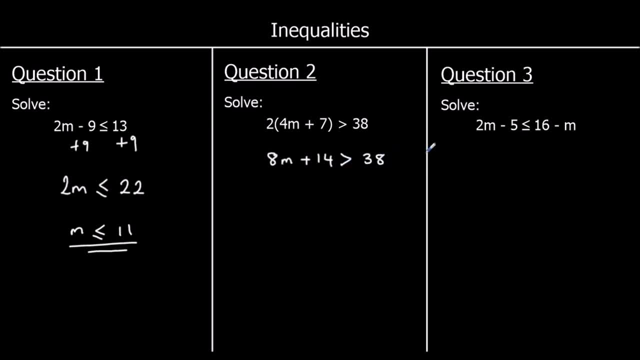 is bigger than 38.. we want m by itself, so we're going to take away 14 from both sides, which leaves us 8m is bigger than 24.. and then, dividing both sides by 8, 24 over 8 is 3.. so m is bigger than 3.. 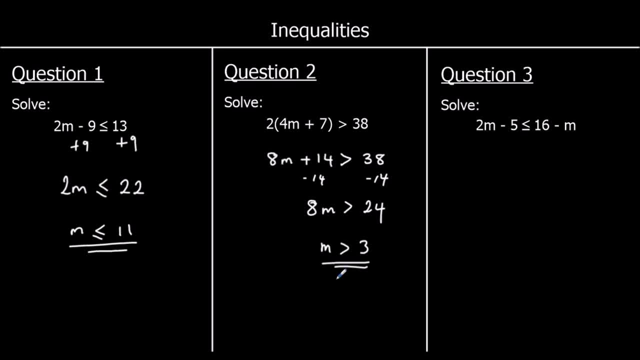 and question three: i've got an m on both sides of the equation. i want to get rid of the smallest one, which is minus 1m, negative 1m, so i'm going to plus 1m to both sides, so i've got 3m. 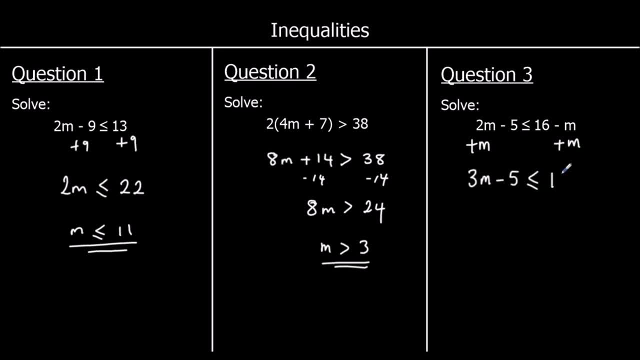 minus 5 is less than or equal to 16. i'm going to plus 5 to both sides: 1., 12., 3., 15., 15., 27., 26., 11., 29.. I've got 3m is less than or equal to 21, and dividing both sides by 3, that leaves me with.